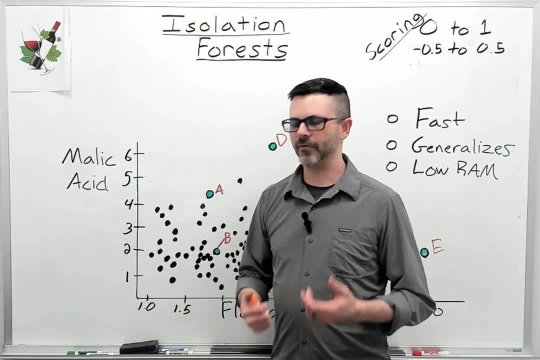 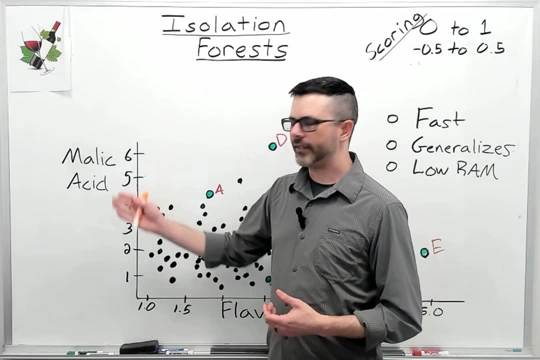 Flavonoids give wine a general mouthfeel and flavor, but too much might not be a good thing. I'm going to use a method to identify anomalies in these two characteristics. It was originally pioneered by Liu Ting and Zhou. That method is isolation forest. 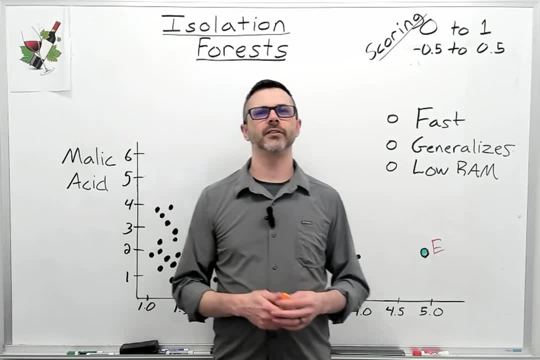 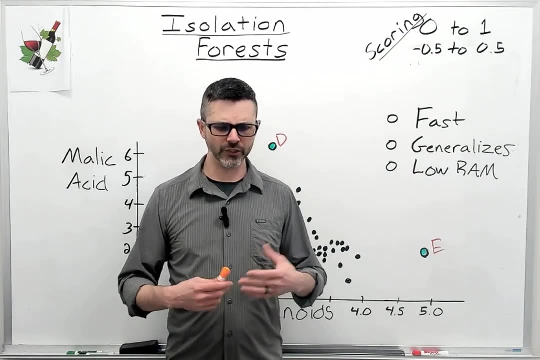 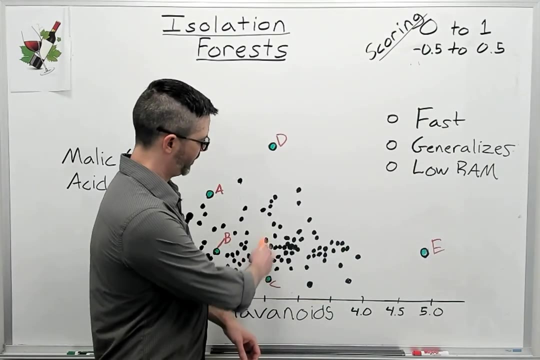 You might've heard of other machine learning methods using the word forest, And there's some similarities, the most common being random forest, which used decision trees under the hood, Which Is a way to separate data out into like categories. In other words, in each group you get a similar group of things that you then 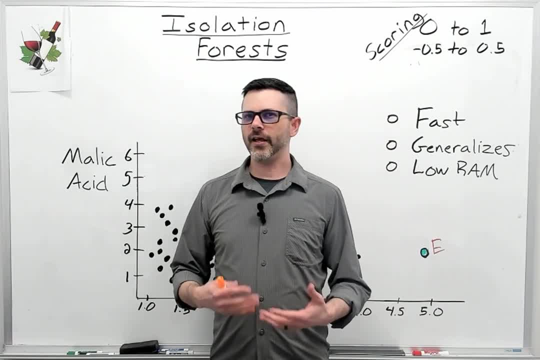 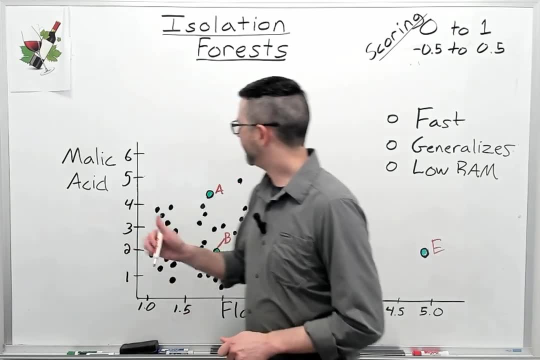 throw a label on and say: you know, these are all one thing. unlike that, an isolation forest seek to separate data completely. It does that using a thing called a binary tree. Just as a quick example, if I had two data points right here and I 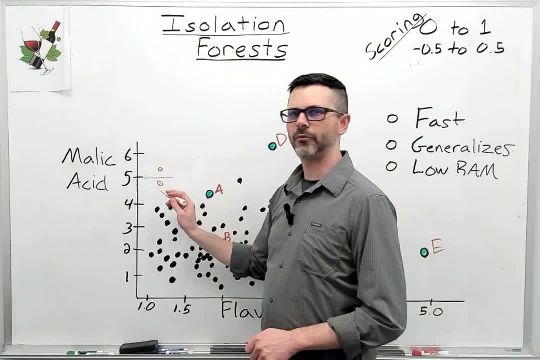 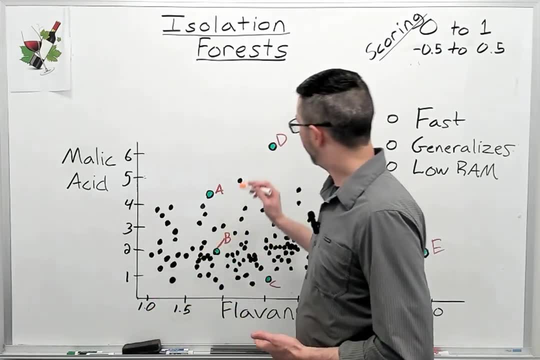 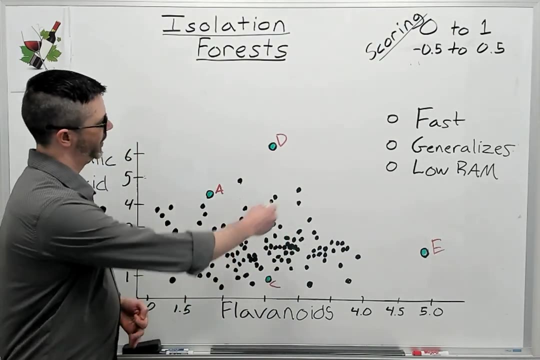 separated at five. on malic acid, these two are separated. Now, if I want to actually apply this to real data, what I'd be looking for is how easy it is to separate a data point from the rest of the data. So if I look at D anywhere between five and six, we'll separate D in one cut. 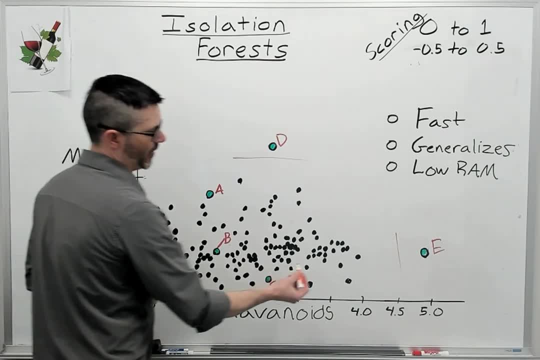 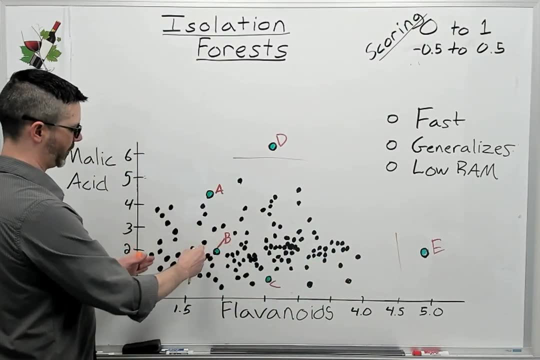 E, similarly at 4.5, is completely separated and that entire range. if we were randomly drawing these cuts, I have a pretty good probability of hitting that, compared to hitting something Over here that separates out a single point. Now another example is a in the middle. here it takes a minimum of two cuts. 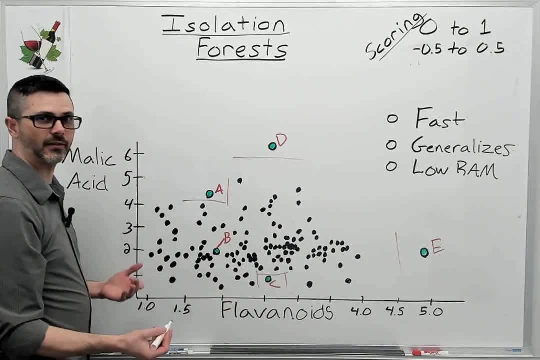 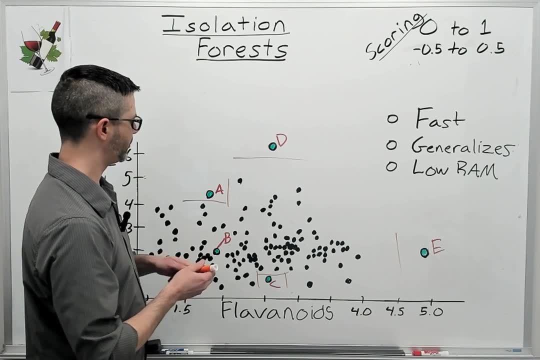 And then, similarly for C, I have to make three cuts to completely separate it from all the data. And then B over here it takes four. I'd have to completely box it into separate it. So we actually write these out. I have a, B, C, D and E. 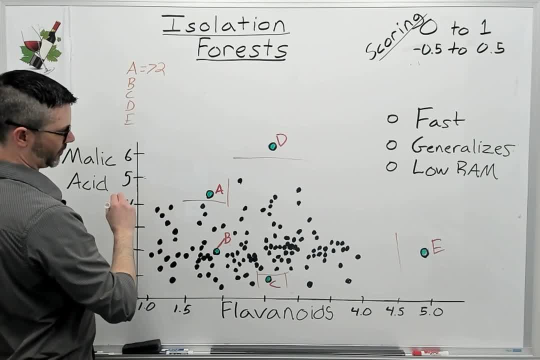 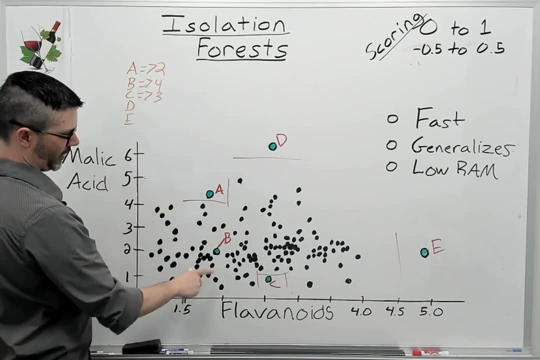 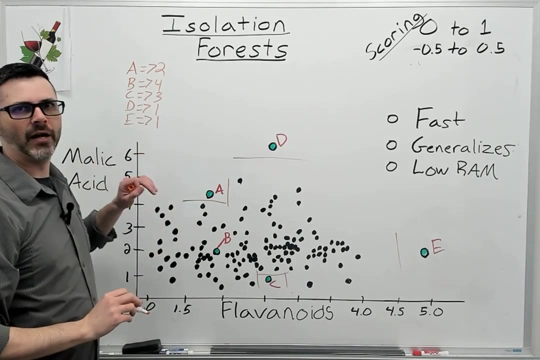 A takes two, B, C, D Takes four, C Takes three, D only takes one and E only takes one, but these are lower bound for this method. In other words, there's not a way to completely isolate any of these.